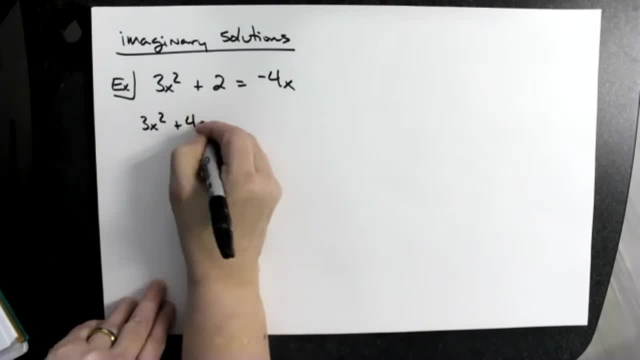 middle. So I'm going to go 3x squared, I'm going to add 4x, because I had to add 4x to both sides to get it moved. Plus 2 equals 0.. All right, at that point, then. now we have our a value, our b value and our c. 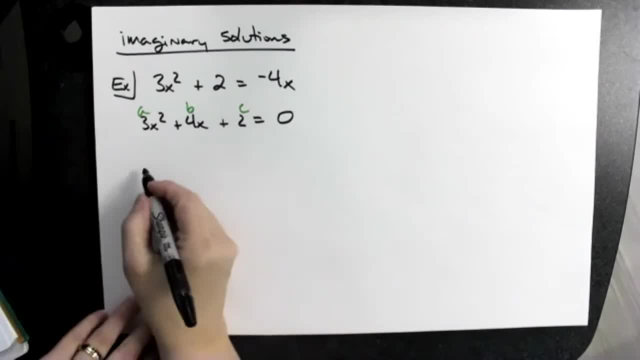 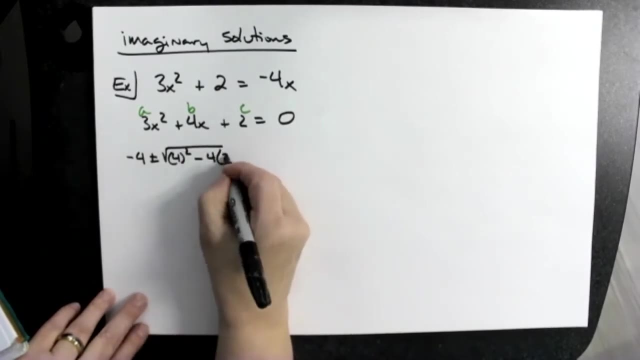 value. Okay, so again we can plug this in. It's basic arithmetic. All right, hopefully by now we've got the formula memorized, so I'm not going to rewrite it. Let's do negative: 4 plus or minus b squared, so 4 squared minus 4ac. 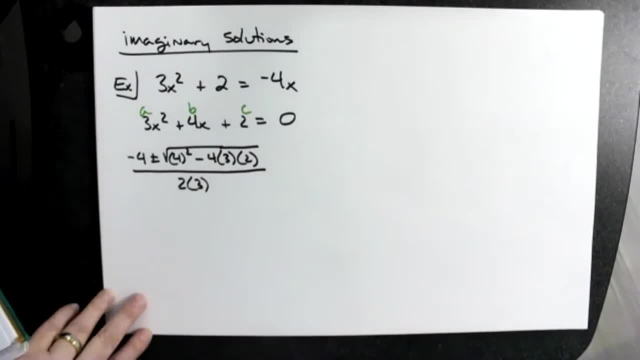 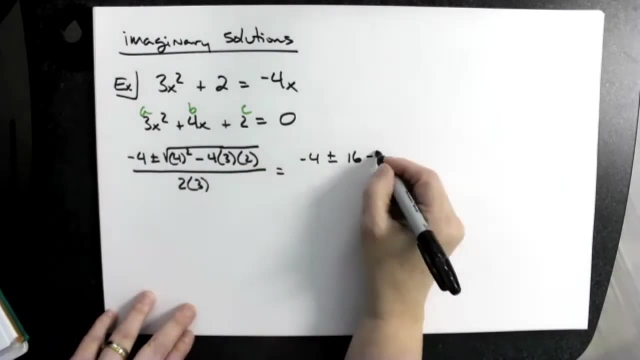 All right, Negative 4 out in front stays put. That's going to be a 16.. All right, now this is going to be minus. whatever this value is right here: 4 times 3 is 12, times 2 is 24.. 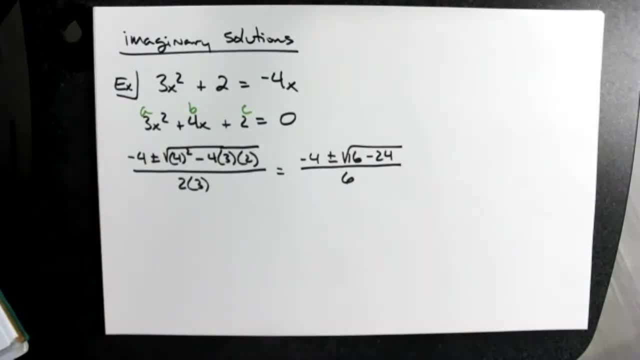 And then all over 6.. All right, so if you can see what's going to happen now, I'm going to get a negative number underneath this square root. Okay, so let's go ahead and do it. Negative 4 plus or minus the square root of a negative 8.. 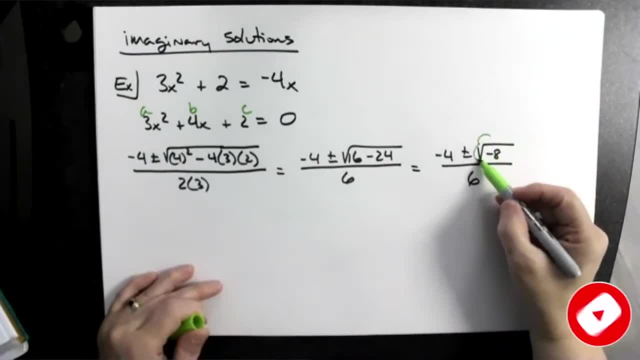 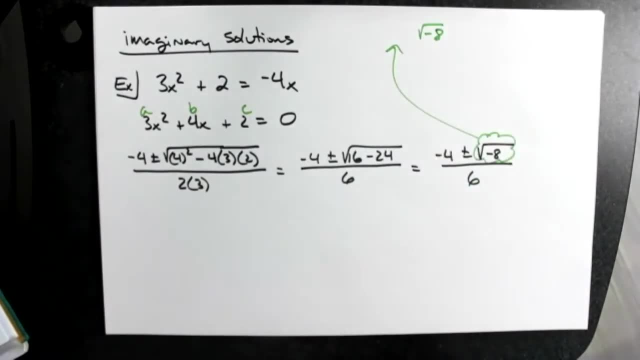 All right up here. let's take this All right and do the work up here. So, square root of a negative 8.. Okay, we did these, I don't know, maybe last week or the week before. All right, let's break that up into the square root of 8 times the square root of a negative 1,. 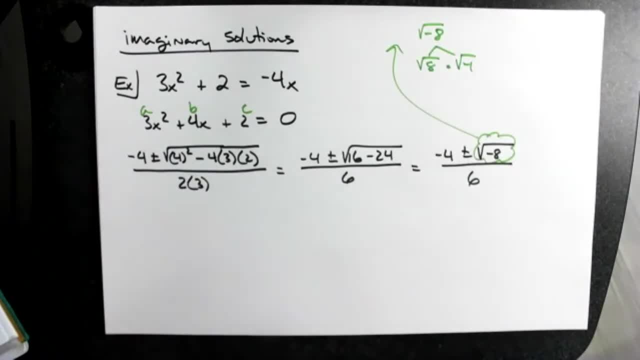 because negative 1 times 8 is going to give me that negative 8.. Get that negative 1 out there by itself, so that we know that square root of negative 1 is going to be an i, because that's going to be our imaginary number. All right, break this up just like we always have. 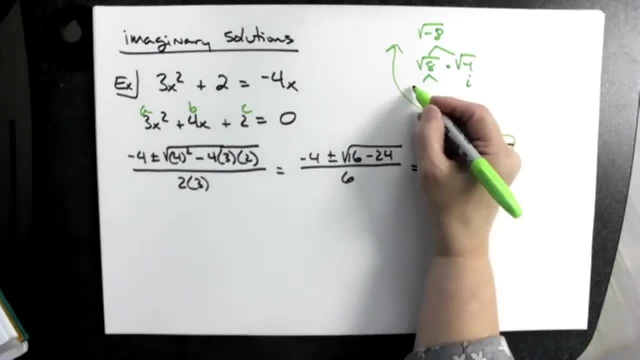 Hopefully, with as much as we've been doing radicals, you've got that one memorized. but if not, square root of 4 times square root of 2.. Biggest perfect square. Okay, so this will be a 2 radical 2.. All right, now we still have to get this i in there somehow. 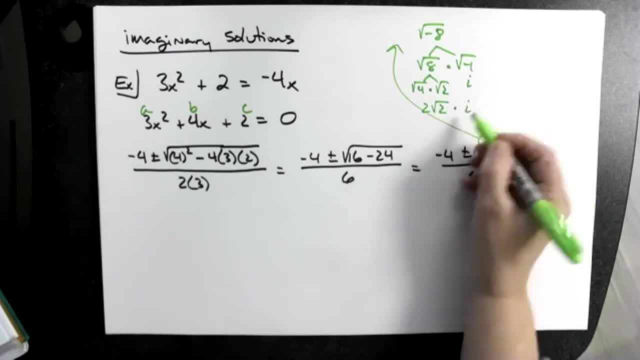 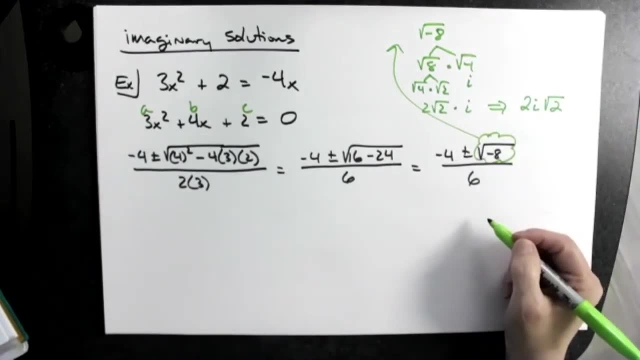 All right. so because it's a multiply, all of this is being multiplied together, So I would write it 2i radical 2 is the way I would write that, Kind of put that i on the inside. okay, All right, now I'm going to.